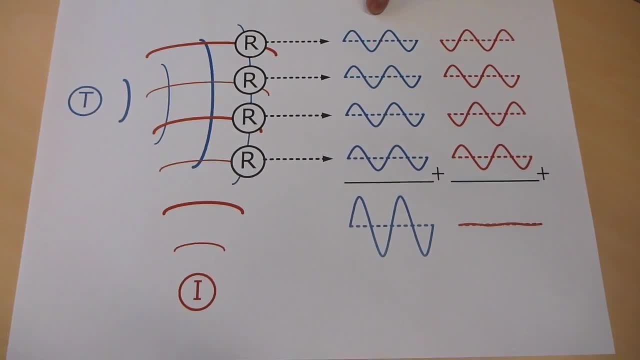 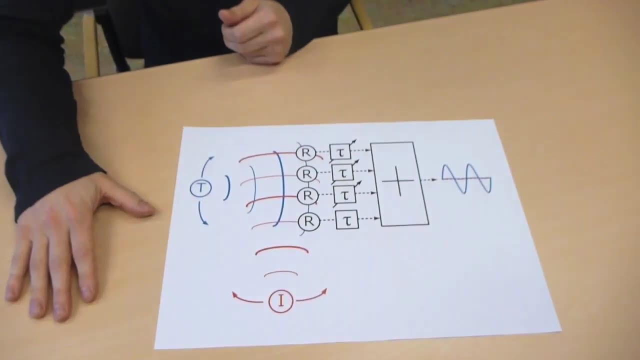 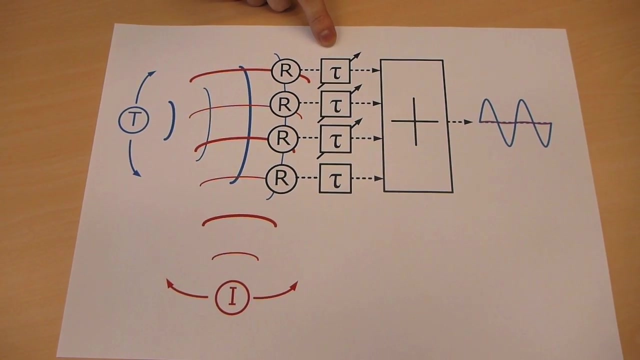 This means that, after summation, our desired signal has maximum amplitude while the interferer is being cancelled. However, if either the desired signal or the interferer is moving, this technique will not work and we have to insert adaptive allays to compensate for the 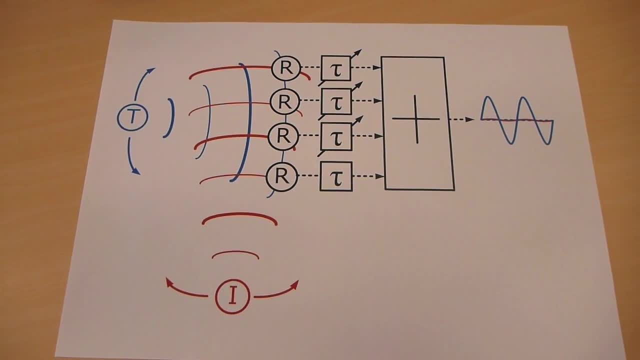 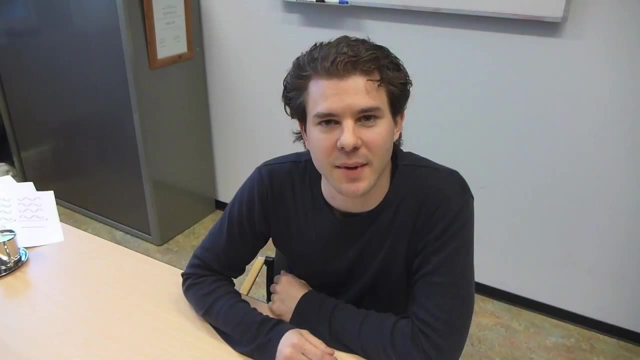 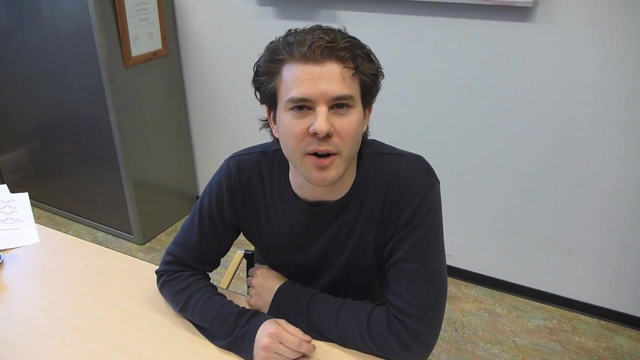 different arrival times of the interferer and the transmitter, So that after summation we still get a cancellation of the interferer and the maximum amplitude of the desired signal. In my research work I have designed a chip in 65 nm CMOS which implements the beamforming 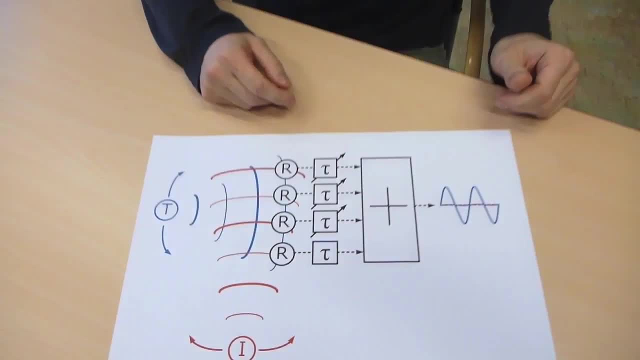 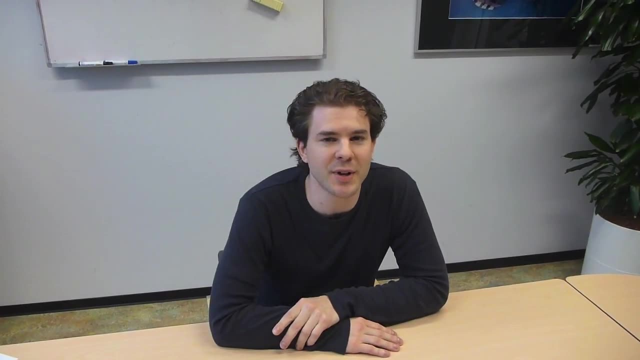 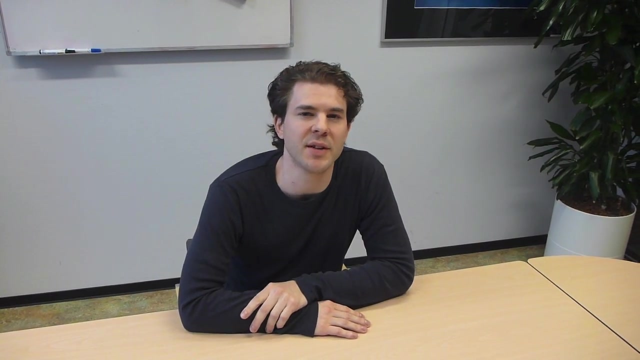 hardware required for this algorithm. In the chip we have implemented our variable delays and the summation needed for beamforming. So to demonstrate you this technique, I have built a setup in the lab using my beamforming chip and real antennas in a real antenna space. 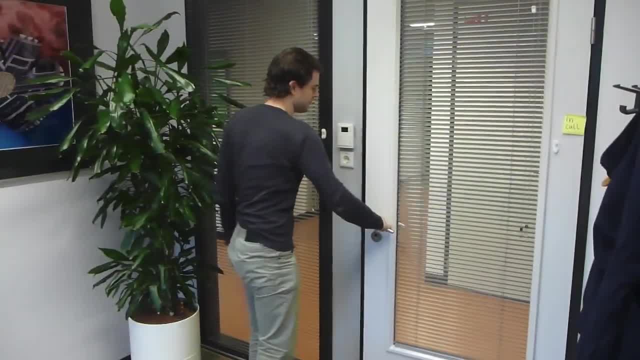 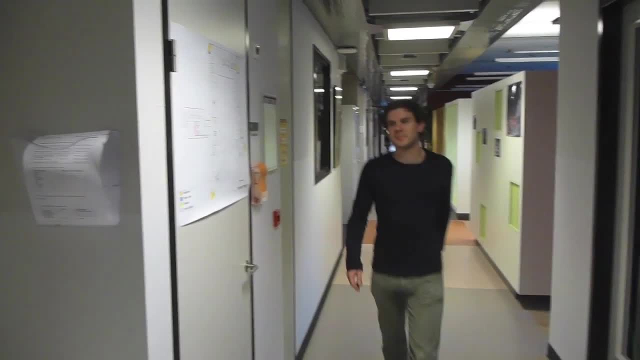 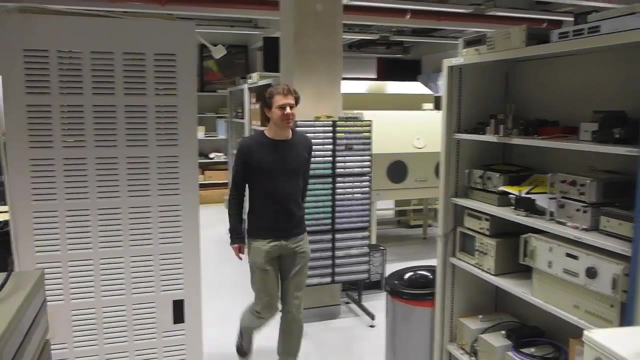 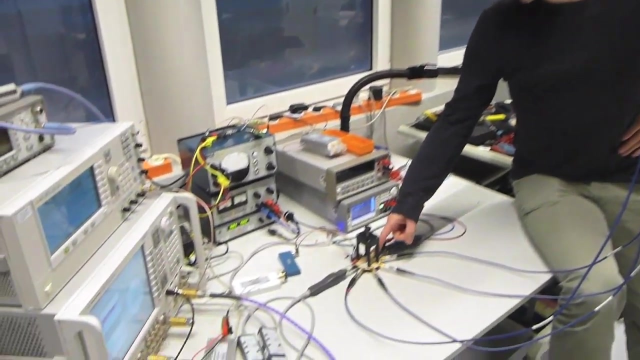 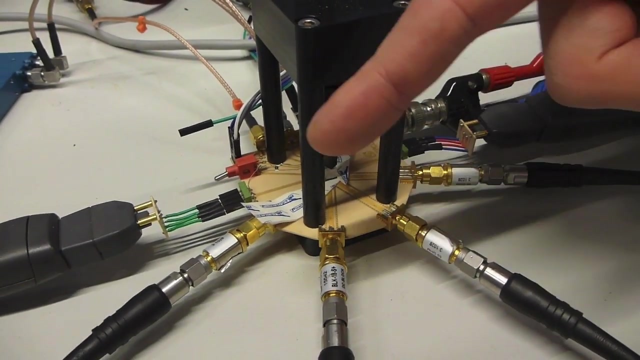 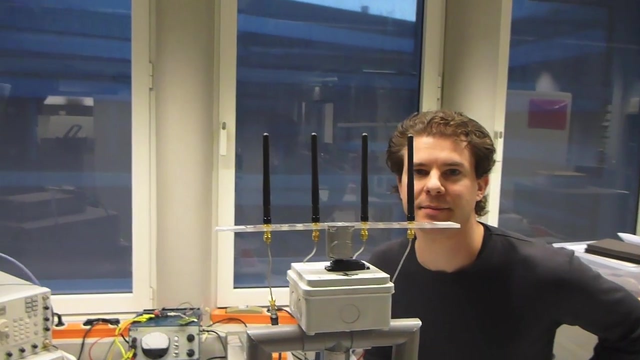 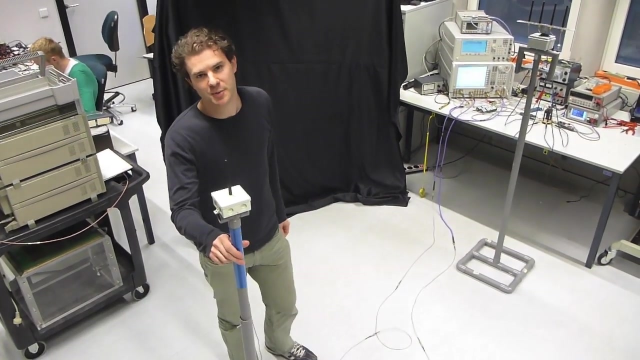 So let's go to the lab. So here we have our setup with the beamforming chip- It is mounted on a PCB- and four inputs which are going to our four antennas here in our antenna array, With our receiving antenna. here we have in our setup also a transmitter with our desired. 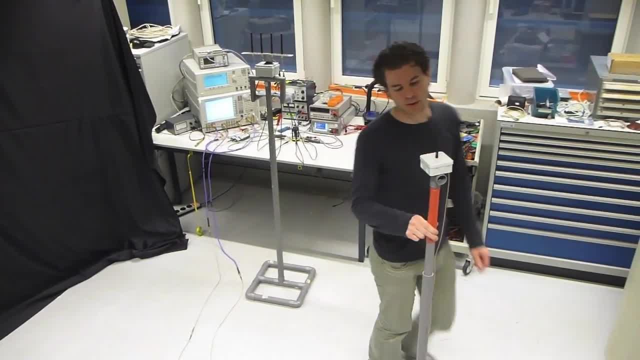 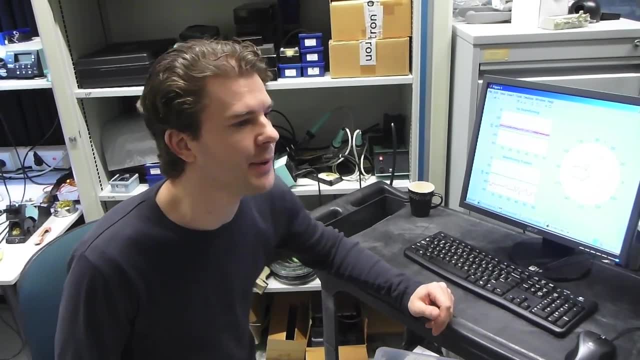 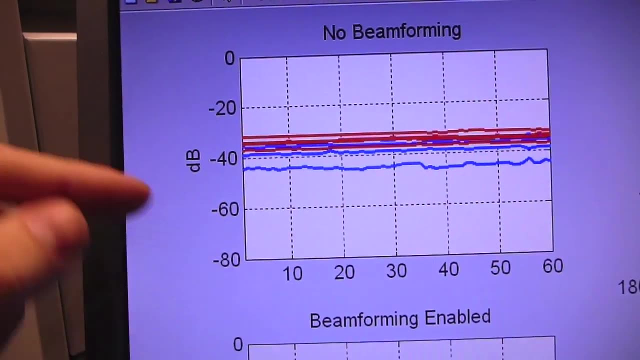 signal and our interferer, which we will cancel out with our beamforming algorithm. Here we see the output of our beamforming chip. Here we see the output of our beamforming chip. Here we see the output of our beamforming algorithm. On the screen we have a plot where we see the power as a function of time, where our 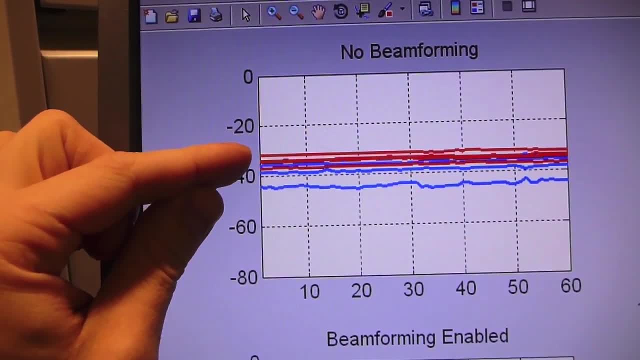 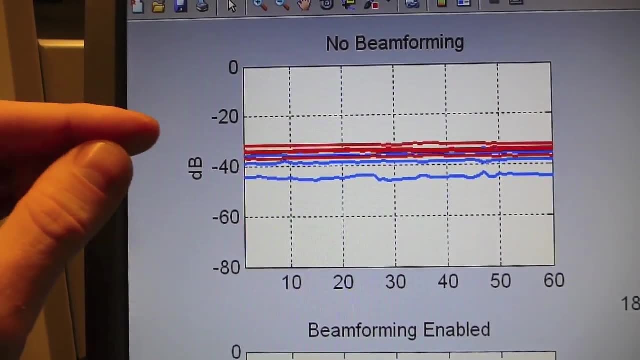 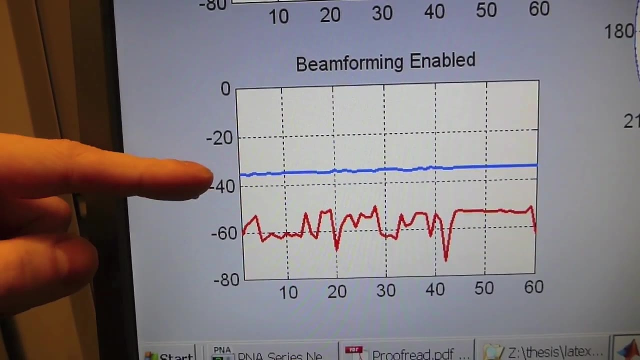 interferer is shown here in four red lines for the four receiver antennas and our desired signal is also in four lines in blue And we see that the interferer is stronger than the desired signal. However, after beamforming we see that the desired signal still has its same strength, while the 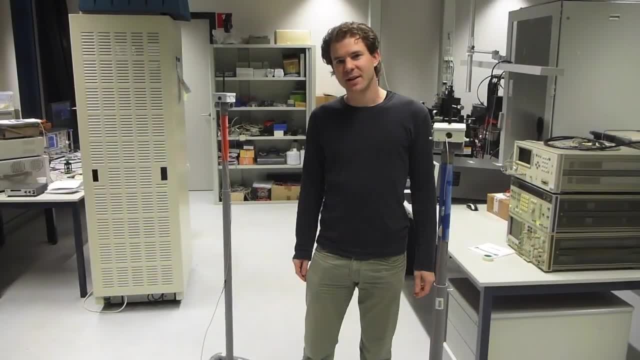 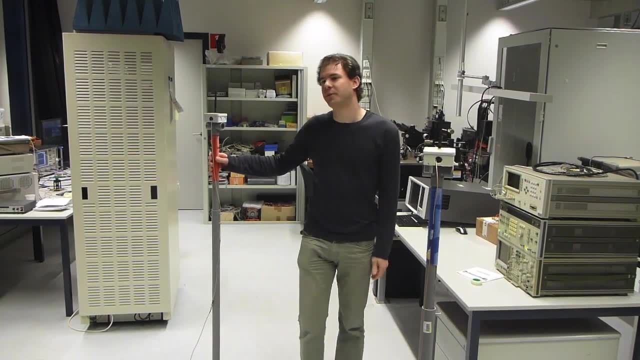 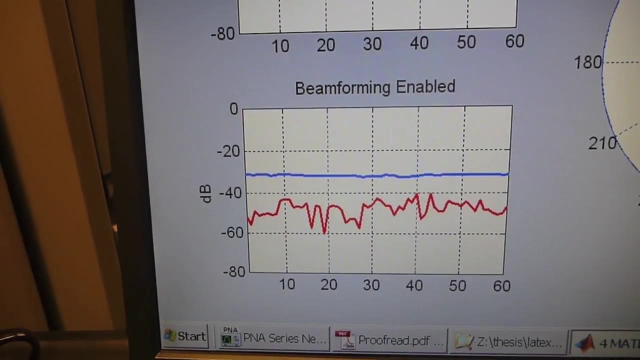 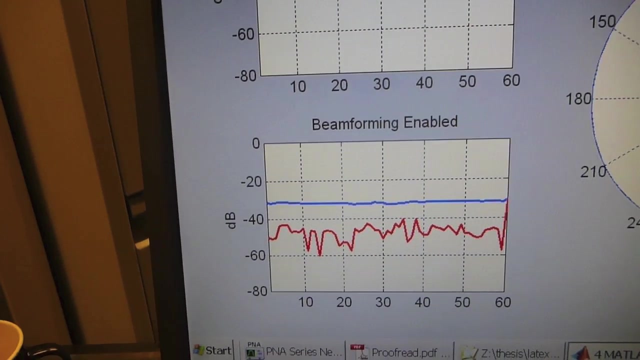 interferer has been suppressed greatly. Now, with our beamforming algorithm, we are receiving our desired signal while suppressing our interferer. However, if we now move the interferer, the cancellation will not be there anymore. So if we move the position of the interferer, we see that the cancellation of the interferer 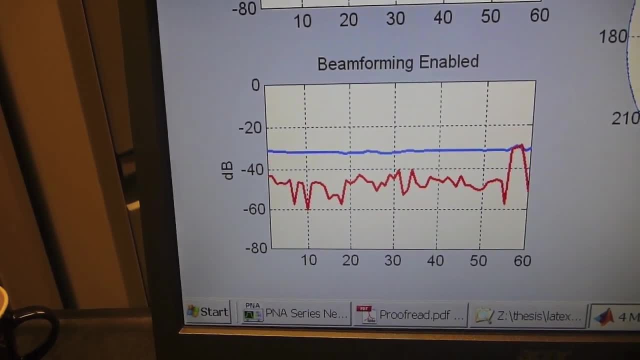 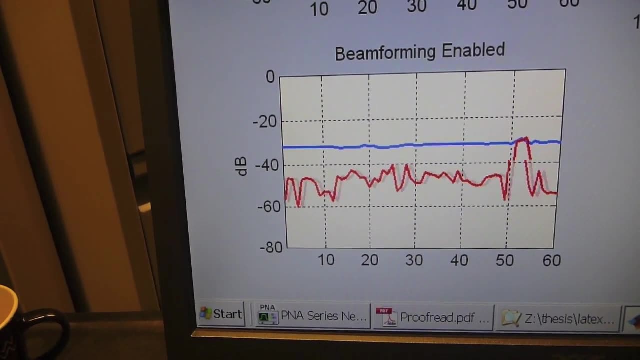 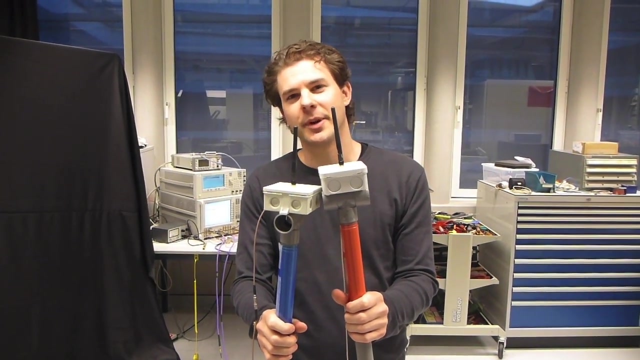 is broken. However, after some settling time, The adaptive algorithm determines a new position and adaptively cancels the interferer again. Even if we put our interferer very close to our desired signal, the beamforming algorithm is still able to suppress the interferer due to the multi-path reflections in a typical 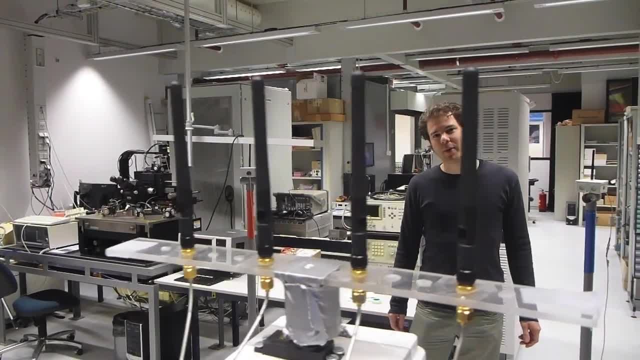 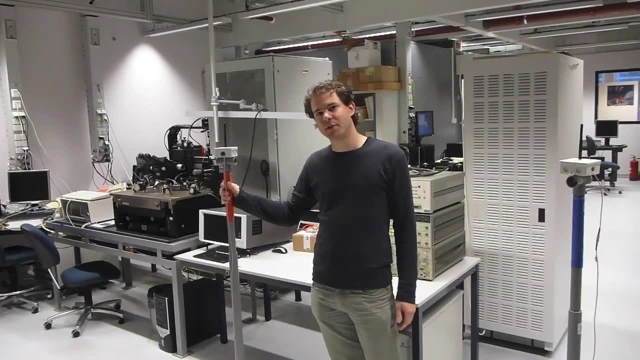 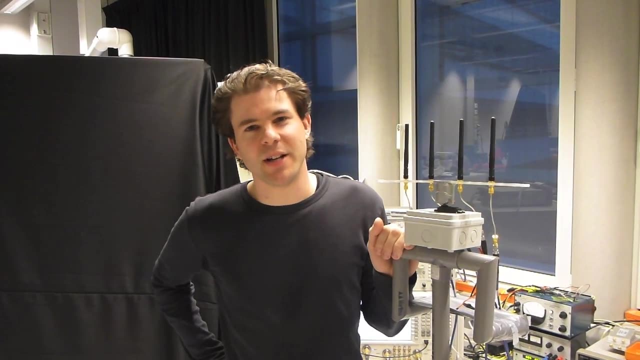 room such as this. Now we have built an array which receives our desired signal and also suppresses our interferer. So with our beamforming algorithm, we can suppress the interferer, which will lead to better and faster mobile internet in the future.